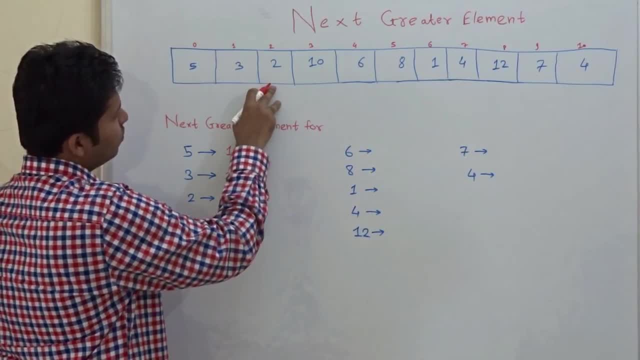 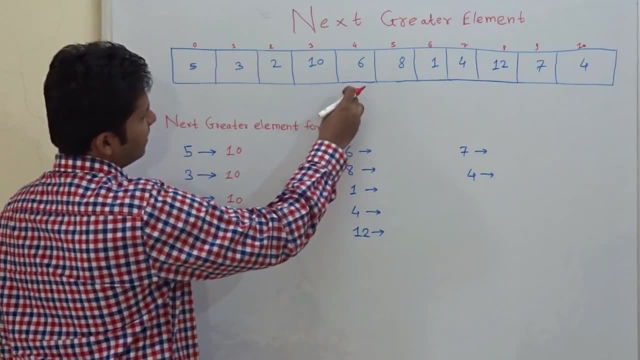 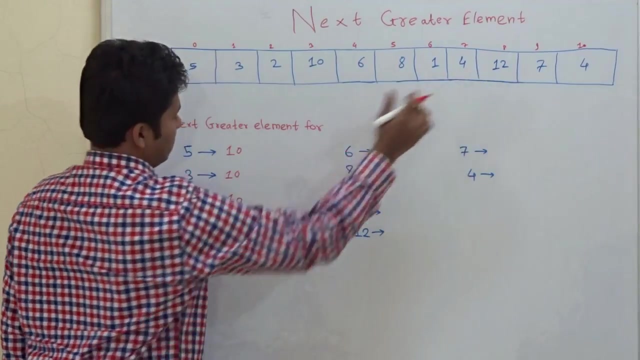 10 is the next greater element For 2, obviously, 10 is the next greater element For 10,. 6 is less than 10.. 8 is less than 10.. 1 is less than 10.. 10, 4 is less than 10,. 12 is greater than 10.. So 12 is the next greater element Now. 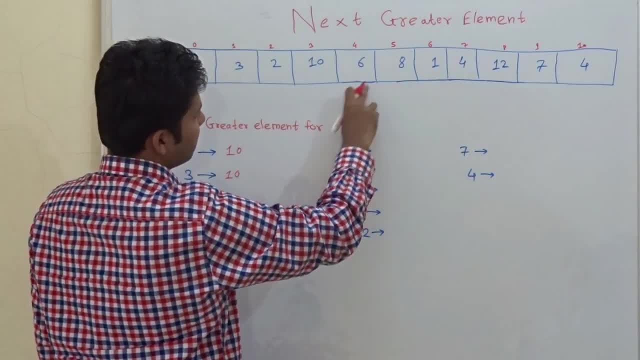 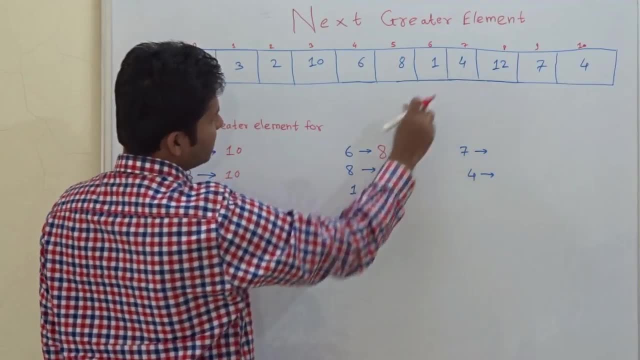 for 6,. 8 is greater than 6.. So 8 is the next greater element For 8,. 1 is less than 8,. 4 is less than 8,. 12 is greater than 8.. So 12 is the next greater element For 1, 4. 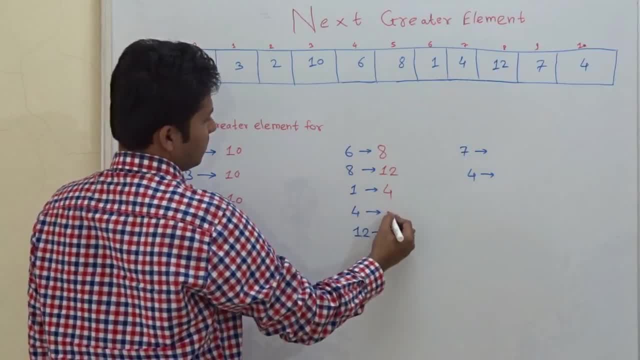 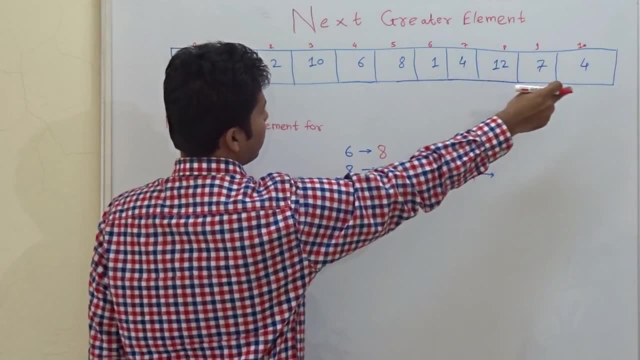 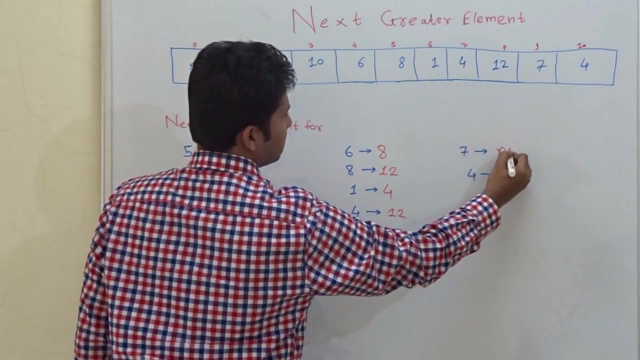 is the next greater element For 4,. 12 is the next greater element For 12,. yes, there is no next greater element for 12 in this array, So there is no next greater element For 7,. there is no next. 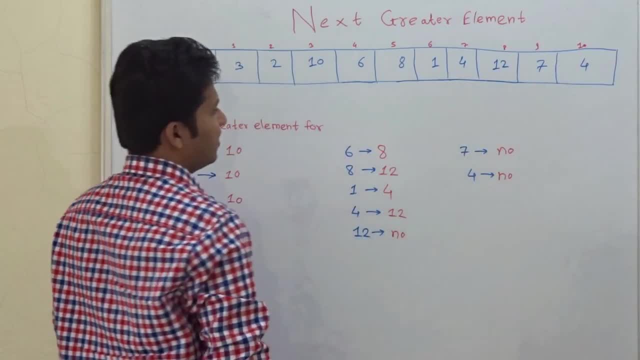 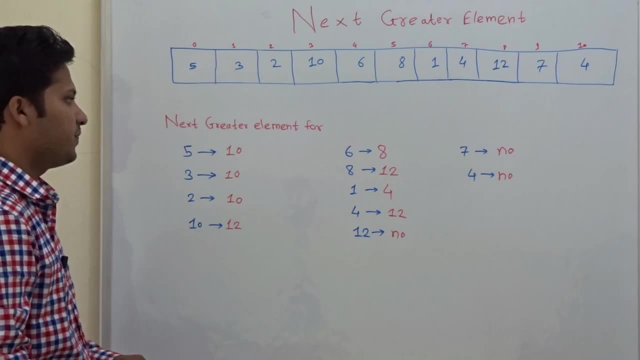 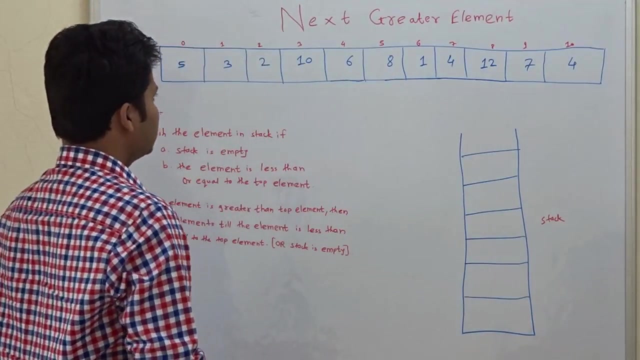 greater element And for 4, there is no next greater element. So this is the way how we find next greater element in the array for each element. now I will tell you the algorithm. now let's see the algorithm. so we are using stack here and I will tell. 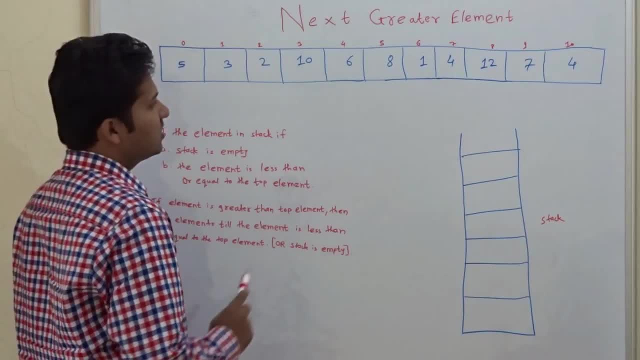 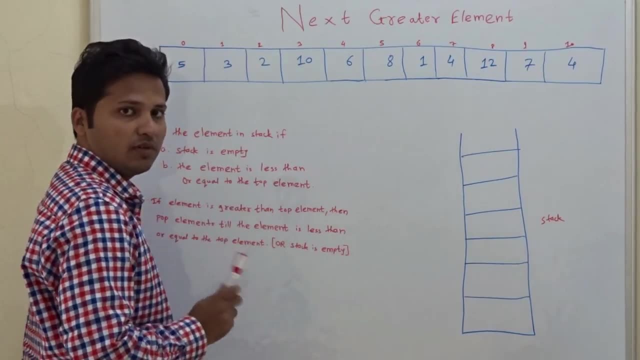 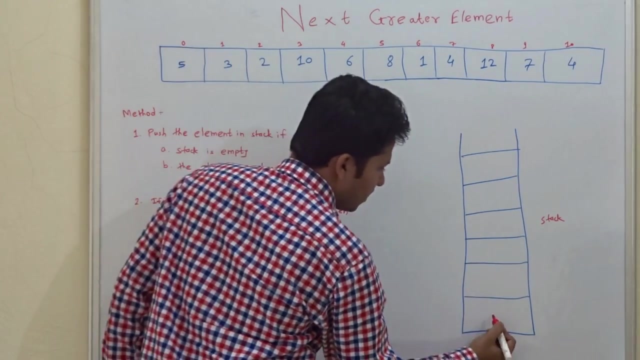 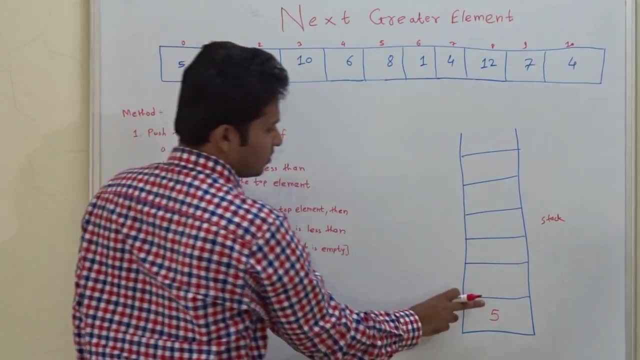 you the method. first we will push the elements into the stack if the top element of the stack is greater than the element which is to be pushed. so now let's see. first we push 5. as the stack is empty, we directly push 5 without checking any condition. then 3, so 3 is less than 5, so we can push 3, 2 is less. 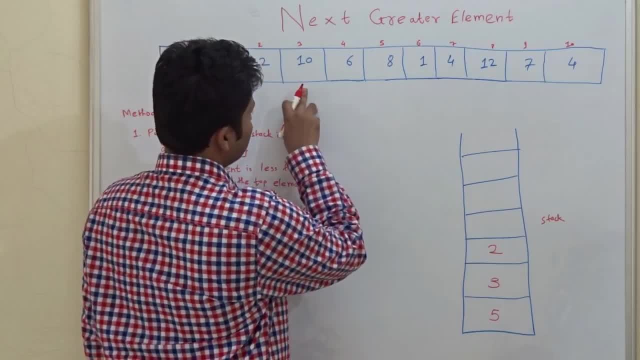 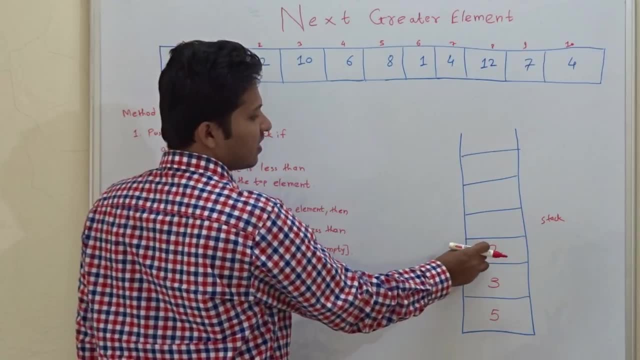 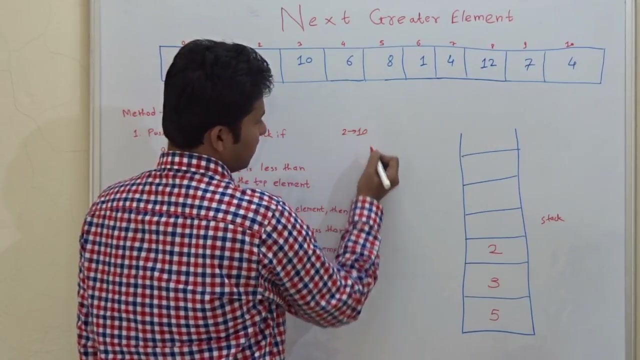 than 3, so we can push 3. you can see 10. 10 is greater than 2, so we cannot push 10. this means that the next greater element for 2 is 10, so next greater element for 2 is 10 and we pop 2, then we check 10. 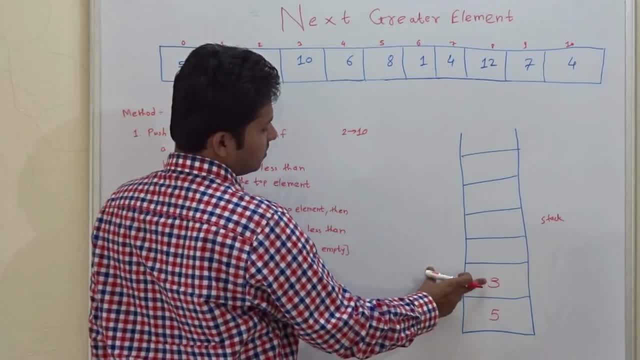 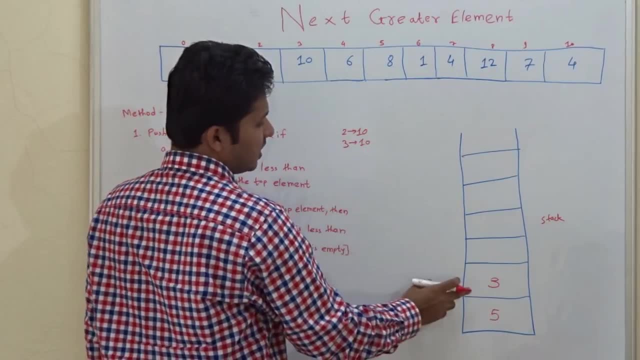 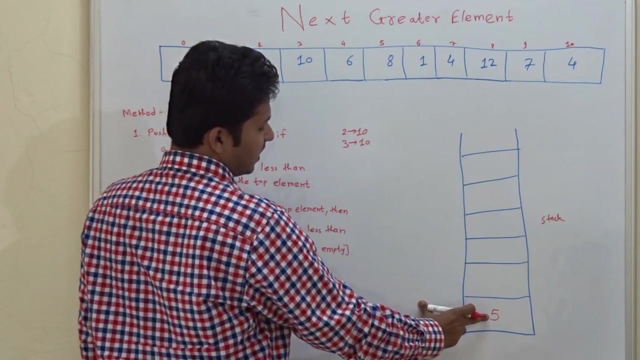 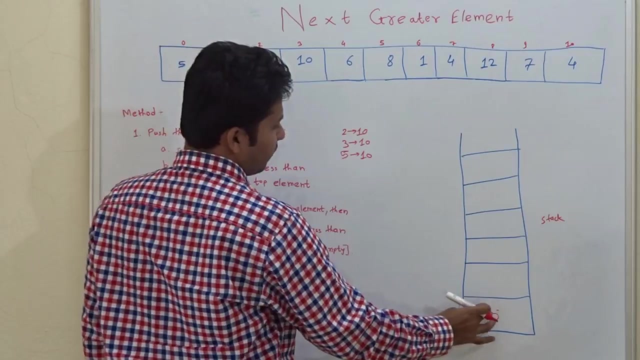 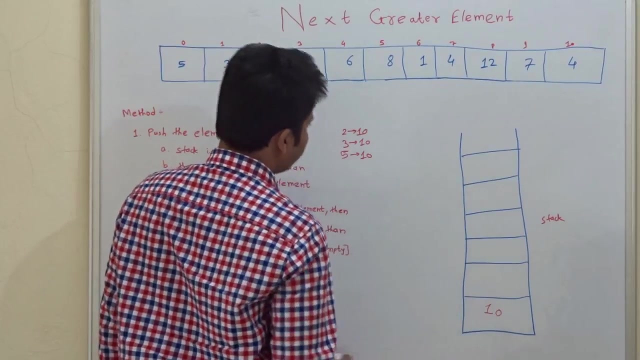 with. we check 10 with 3, so 10 is greater than 3. so the next greater element for 3 is 10 and we pop 3. we check 10 with 5, so the next greater element for 5 is 10 and we pop 5. as the stack is empty, now we push 10. now let's. 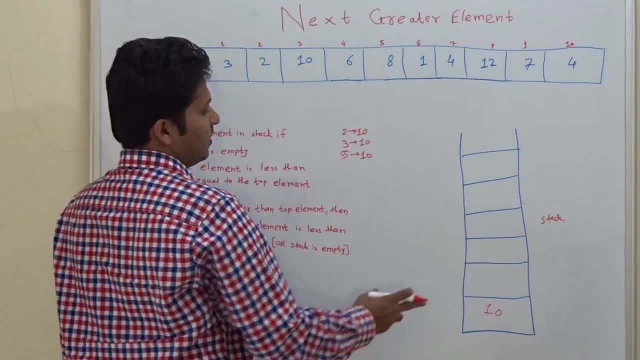 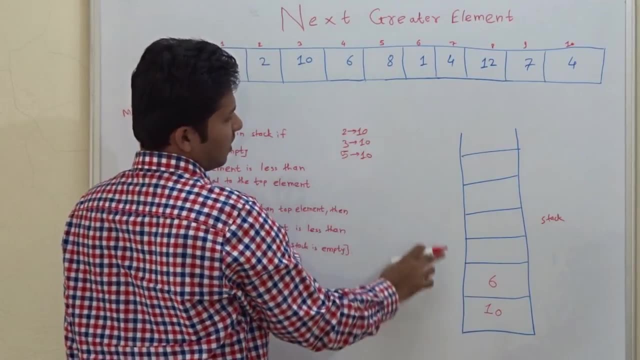 go to the next element, 6, so 6 is greater than 3, so 10 is greater than 3. so we go to the next element, 6, so 6 is greater than 3, so 10 is greater than 3. so we push 6, then 8. 8 is greater than 6. this means that next greater element for 6 is: 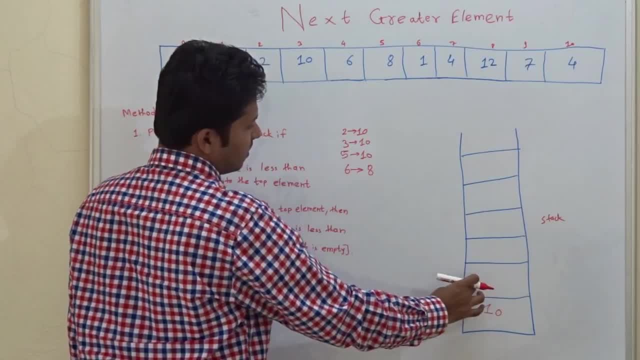 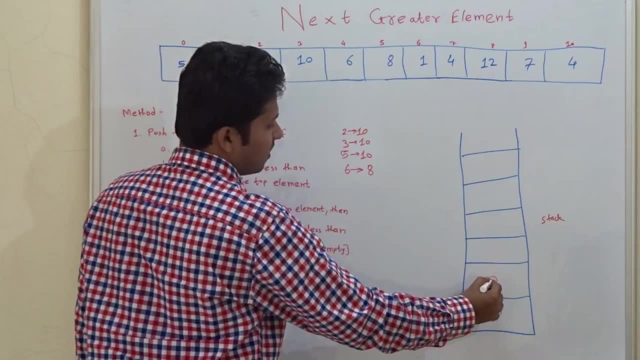 8 and we pop 6. now we check 8 with 10: yes, it is less than 10, so we can push 8. so let's see 1: 1 is less than 8, so we. so let's see 1: 1 is less than 8, so we. 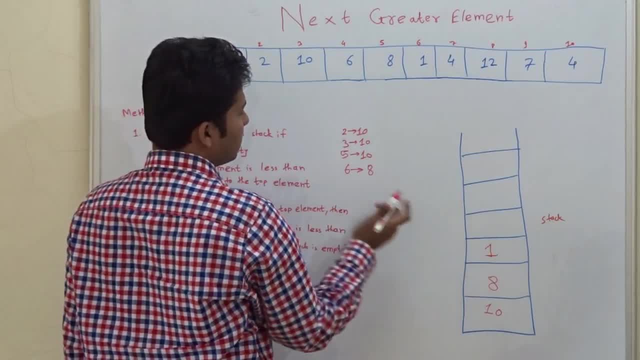 so let's see: 1: 1 is less than 8, so we can push 1 4. 4 is greater than 1, so the can push 1 4. 4 is greater than 1, so the can push 1 4. 4 is greater than 1, so the next greater element for 1 is 4, and we. 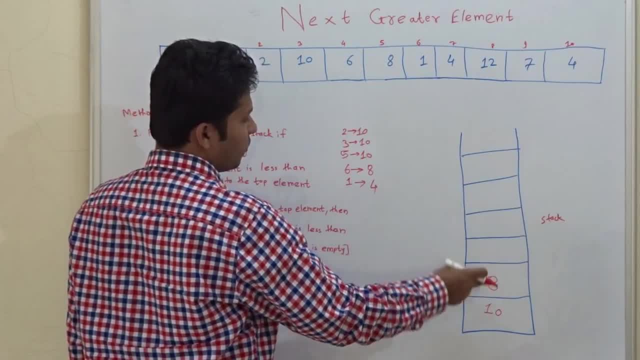 next greater element for 1 is 4 and we next greater element for 1 is 4 and we pop 1. now. we check 4 with 8. 4 is less. pop 1 now. we check 4 with 8: 4 is less. 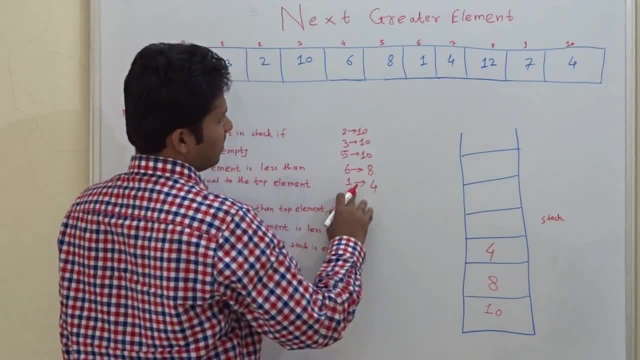 pop 1. now we check 4 with 8: 4 is less than 8, so we push 4. here now 12: 12 is than 8, so we push 4. here now 12: 12 is than 8, so we push 4. here now 12: 12 is greater than 4, so the next greater. 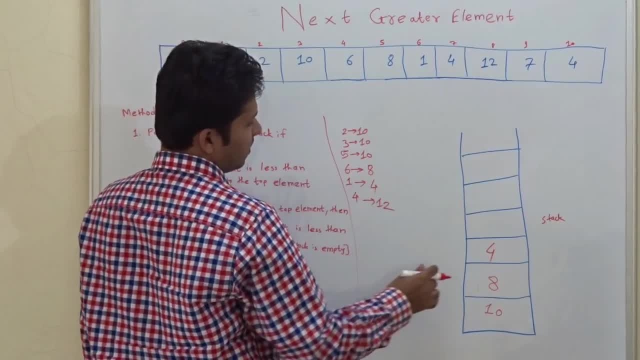 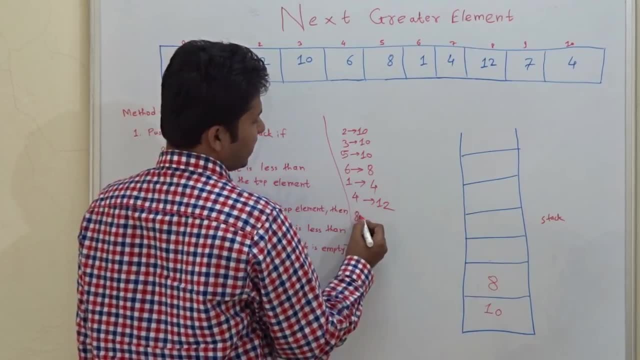 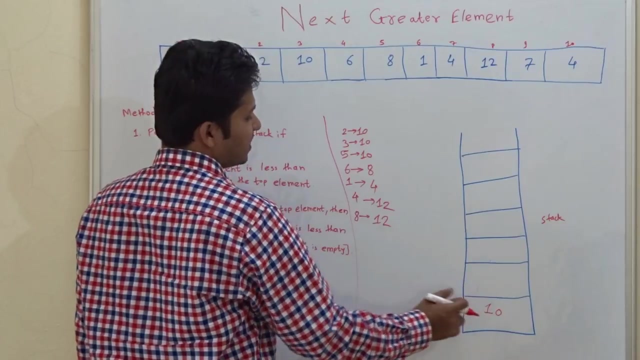 greater than 4. so the next greater greater than 4. so the next greater element for 4 is 12 and we pop 4 element for 4 is 12 and we pop 4, 12 is greater than 8, so the next greater element for 8 is 12 and we pop 8,: 12 is greater. 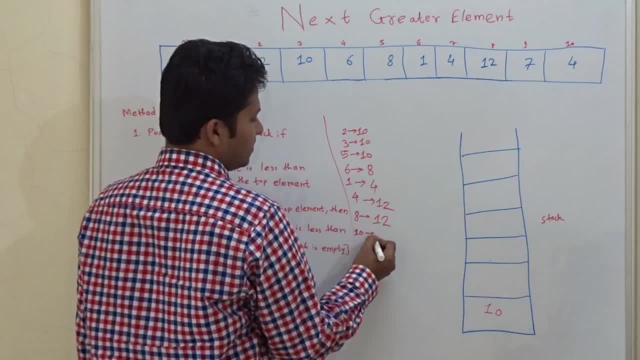 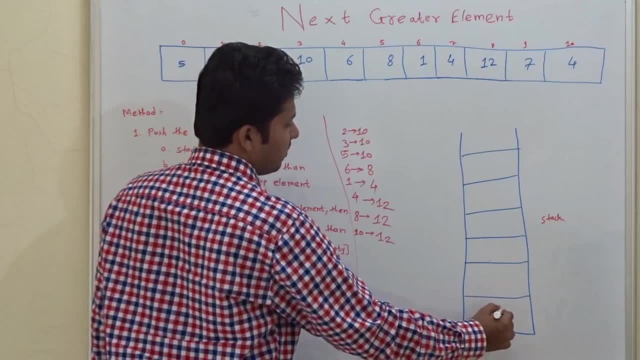 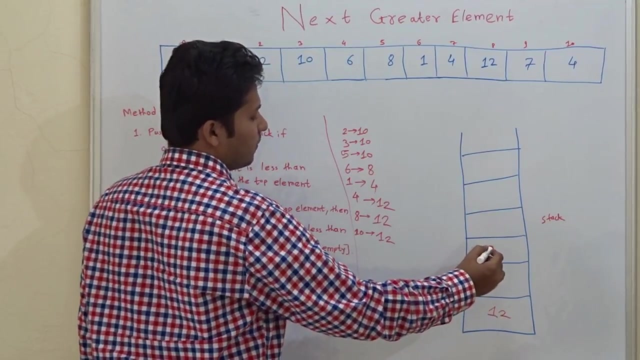 than 10, so the next greater element for 10 is 12, and we pop 10,. now, as the stack is empty, we push 12, now. 7, 7 is less than 12, so we push 7, 4, 4 is less than 7,, so we push.